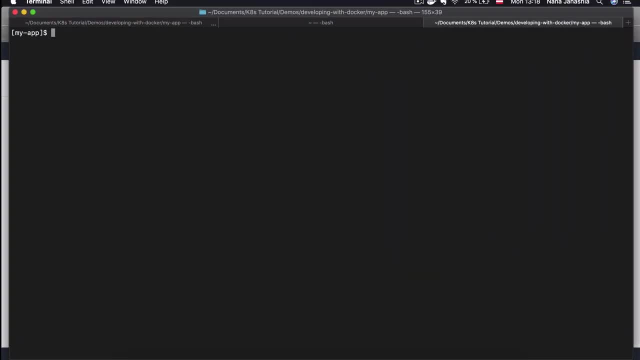 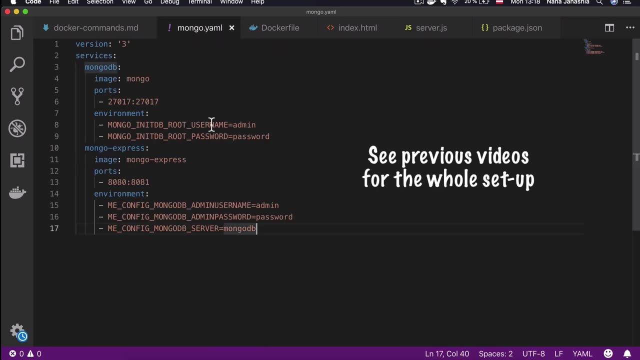 So let's see actually how that would work. So usually again, you have developed your application, Your Done with it and you have created your own Docker image. right now, in order to start an application on development server, you would need all the containers that make up that application environment. 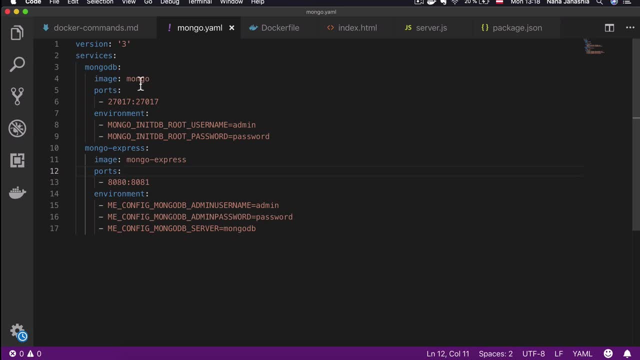 OK, so we have a MongoDB and Mongo Express already, So what we are going to do is here we're going to add a new container in the list, which is going to be our Own image. So let's go ahead and copy the image from our repository. 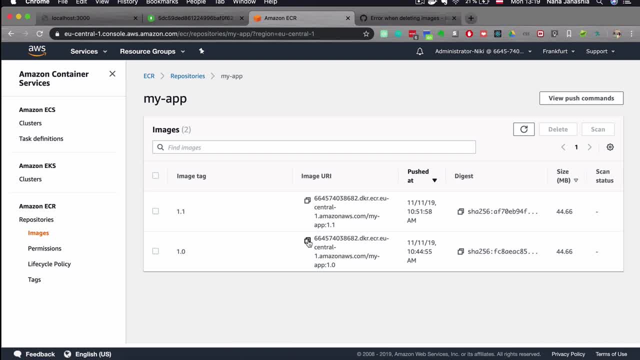 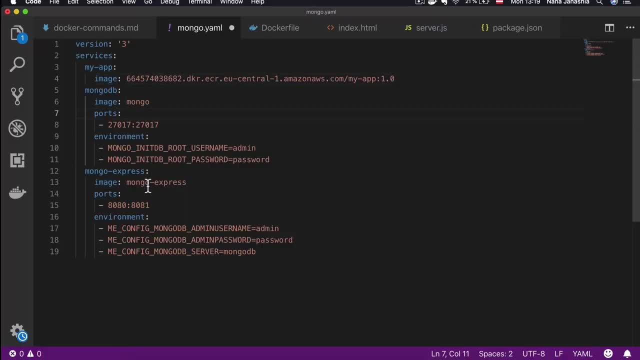 So let's actually use the one point zero. So again, remember we said that this image name is a shortcut for having a Docker dot IO, dot library, slash Mongo With like a specific version. So instead of that, because we are pulling these images from a Docker hub, we can actually skip that repository domain in front of the images. 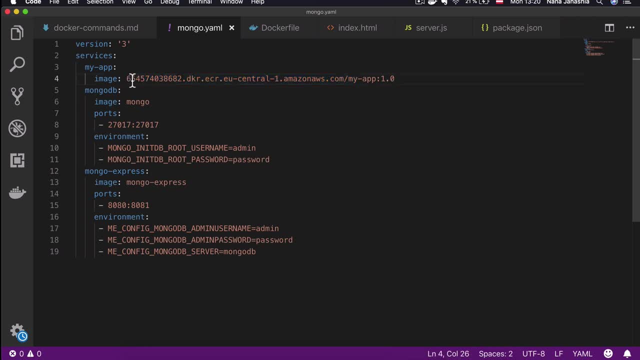 But here because we are pulling it from a private repository. So if we were to specify our image like this, Docker will think that our image resides on Docker hub. So we try to pull it from Docker hub and of course it won't find it, because we have to tell Docker. 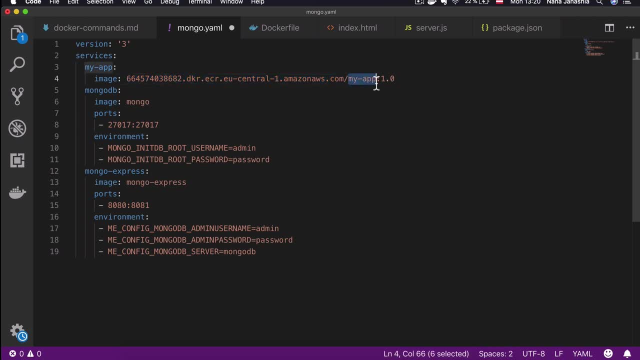 Go and look at this repository with this repository name and this take And, of course, in order to be able to pull this image or the Docker composed, to be able to pull this image, the environment where you executing this Docker compose file has to be logged into a Docker repository. 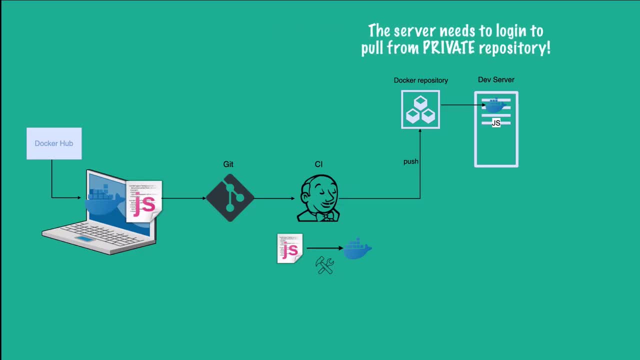 So here, as the development server has to pull the image from the repository, what we would need to do on the development server is actually do a Docker log in Before We execute the Docker compose, and obviously you don't need a Docker log in for Docker hub. 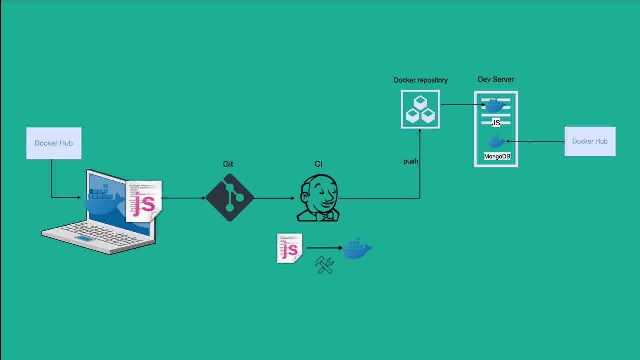 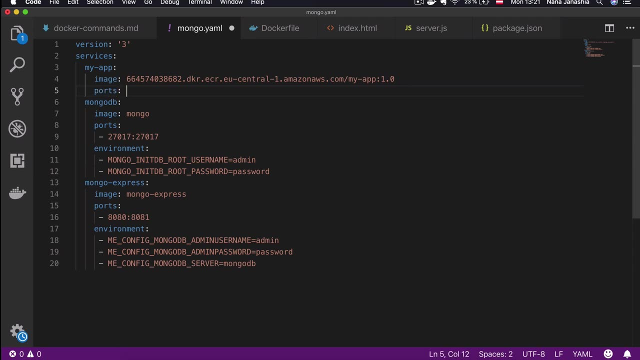 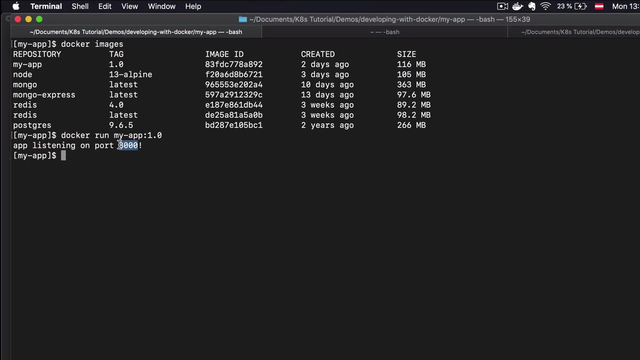 Those Mongo images will be pulled freely. OK, so the next thing that we have to configure are the ports, because obviously we want to open the ports. If we go back, we see that our application runs on Port 3000, so the port of the container, or where the container is listening. 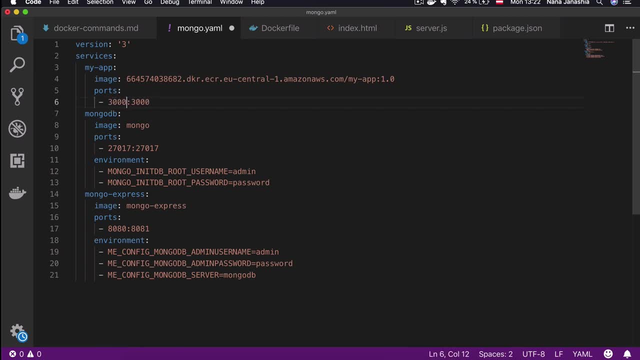 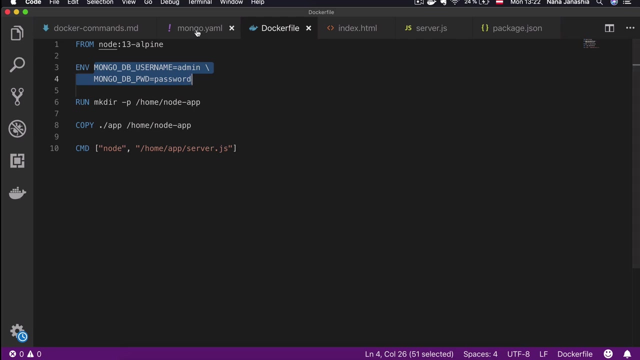 On is three thousand and here we can open the port on the host machine. so it's going to be three thousand. map to three thousand. We have actually the environment variables inside of the Docker file, but obviously we could have configured them in the Docker compose just like this. 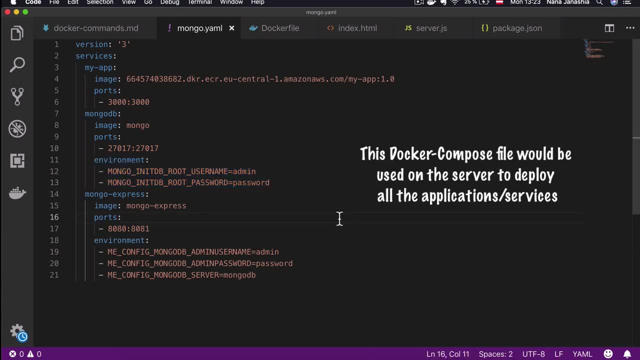 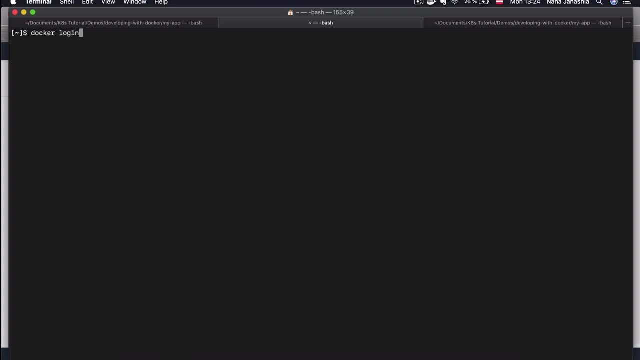 So it's an alternative. so this will be a complete Docker compose file that will be used on the development server To Deploy all the all the applications inside. So again, if we're trying to simulate a development server, the first step will be to do the Docker log in. 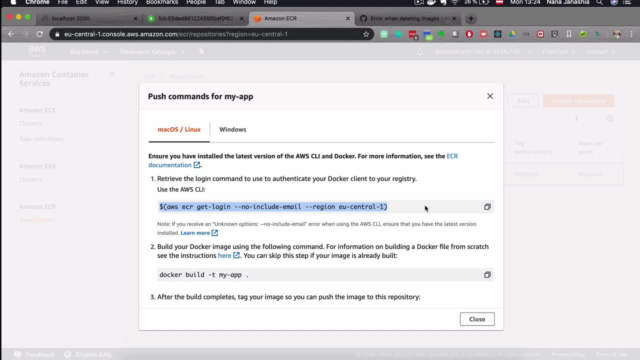 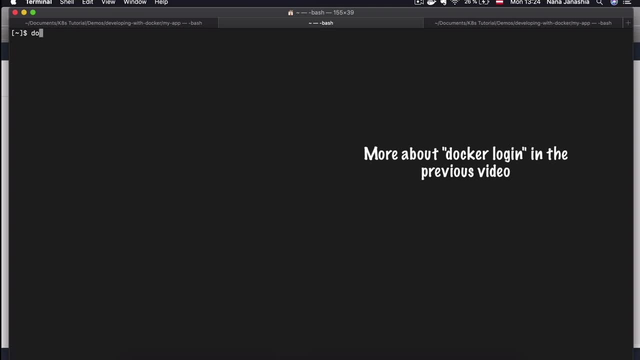 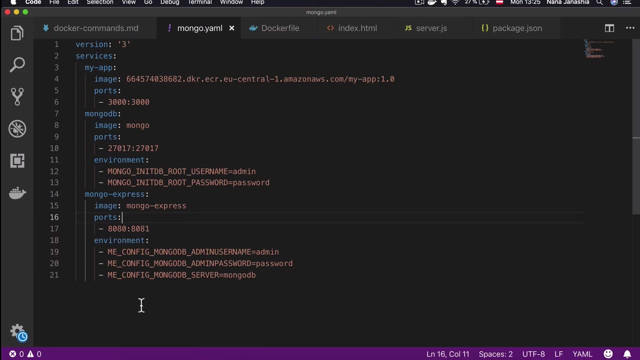 In this case you have this on command for logging into the repository, which I have done already in this terminal. So the next step is to have the Docker compose file available on this development server. because we have to execute the Docker Compose file, because we're simulating here. the way I would do it is: I'm going to create a mongo yaml file in the current directory where I am. I'm going to copy this. 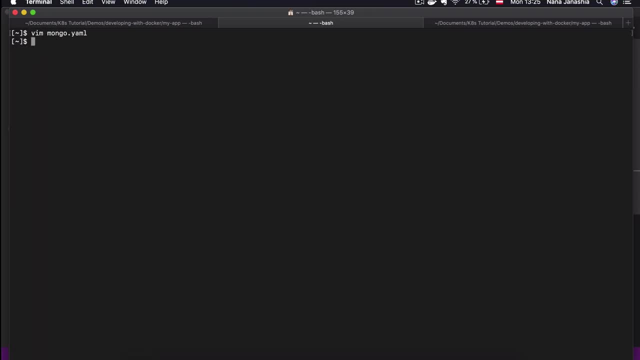 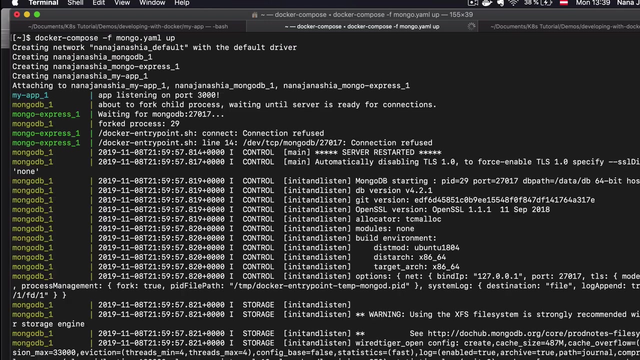 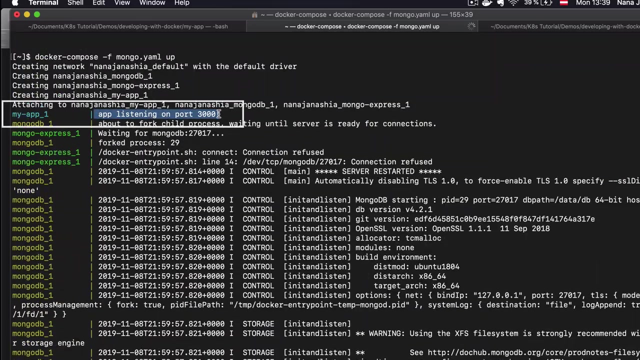 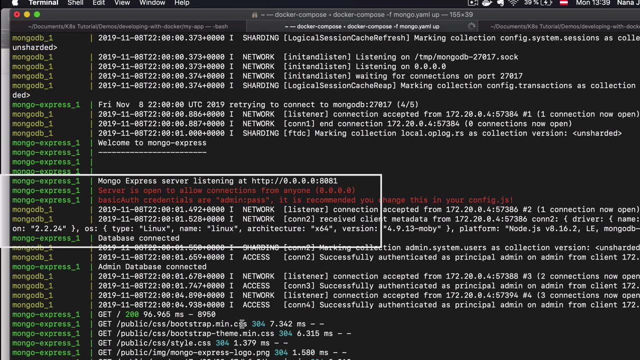 And safe. So now I have my mongo yaml file and now we can start all three containers using monger Docker, compose command Minus F Up, And here we see that it started on three thousand, and MongoDB and express started as well. So let's check again now. 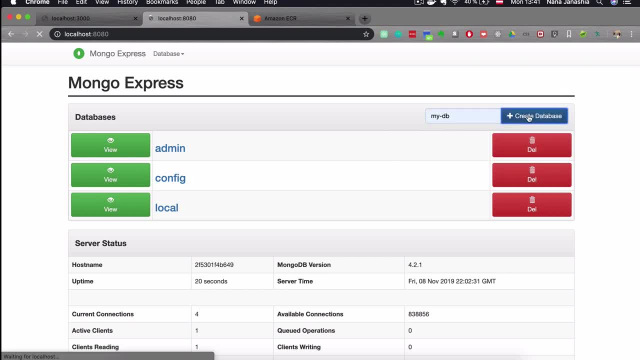 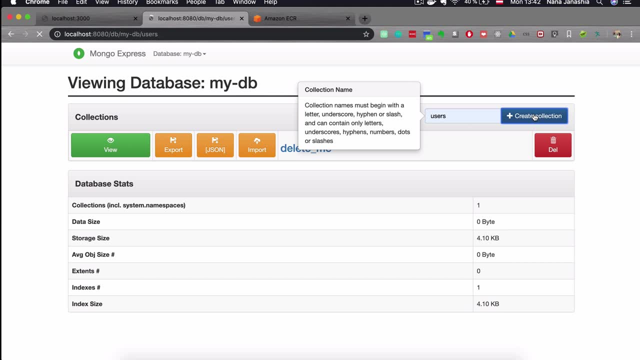 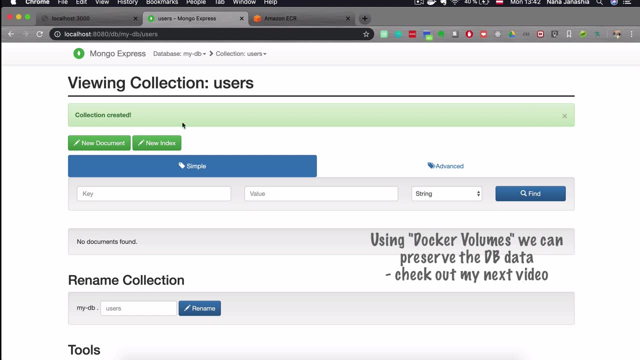 And here we saw, the database is lost every time we recreate a container, And of course that's not good. And we're going to learn how to preserve the database data between the container restarts using Docker volumes in the later tutorials, because this is not an ideal state. 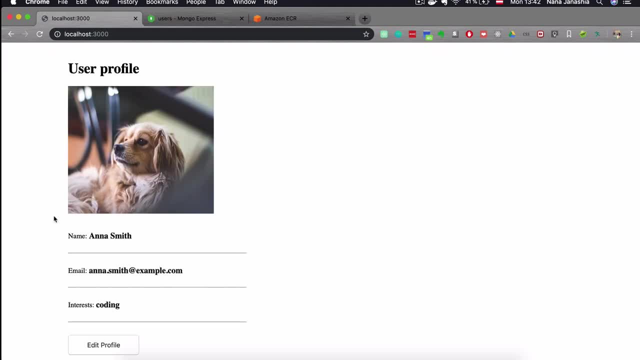 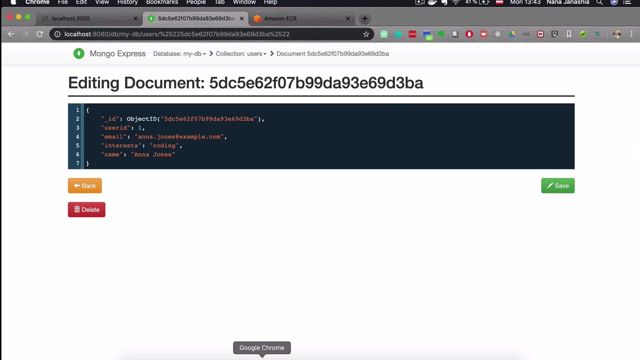 OK, so now that we have the database in a collection, let's actually refresh in. our application works as well. Let's check, Let's refresh this one as well. and there is actually one thing that I needed to change in the code to connect- no Jess- with MongoDB. 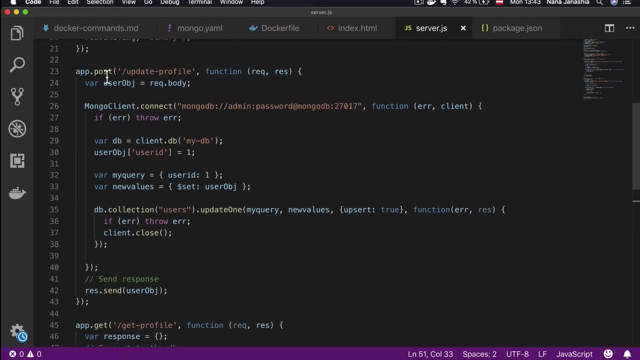 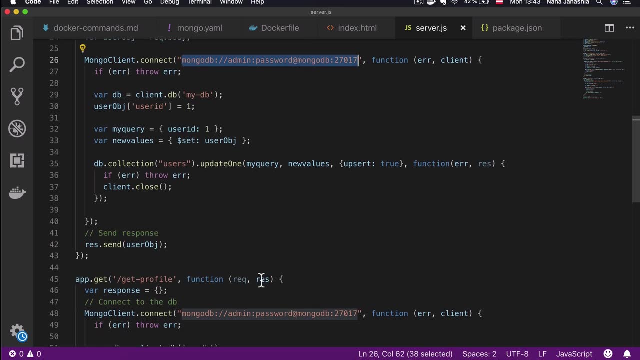 So let's actually go and look at that. So this is my, these are my handlers. you know no, Jess, where I connect to the MongoDB database. So the your eyes are the same, and what I changed here is that it was a local host before. 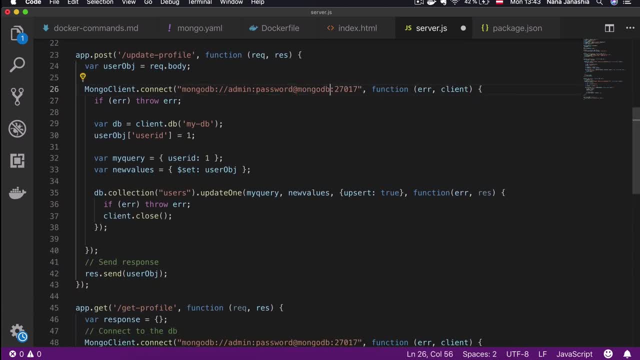 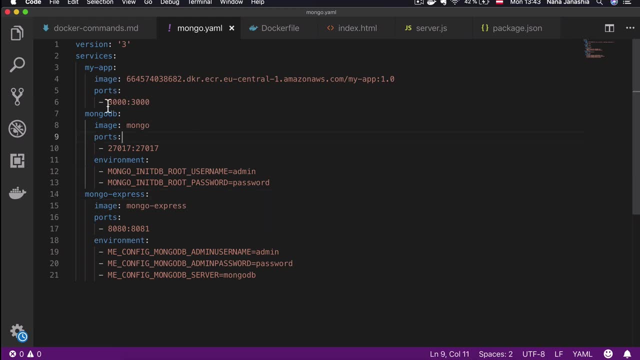 So instead of local host, I changed it to MongoDB, because this actually is a name of the container or of the service that we specify here. So this actually leads back to the Docker network and how Docker compose takes care of it. is that in the your eye? or when I connect one application in a Docker container with another one in another container, I don't have to use this local host? 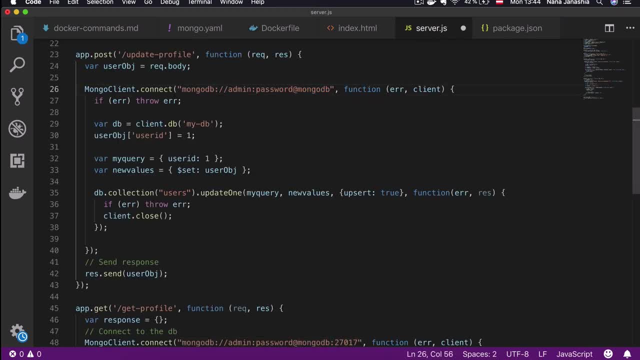 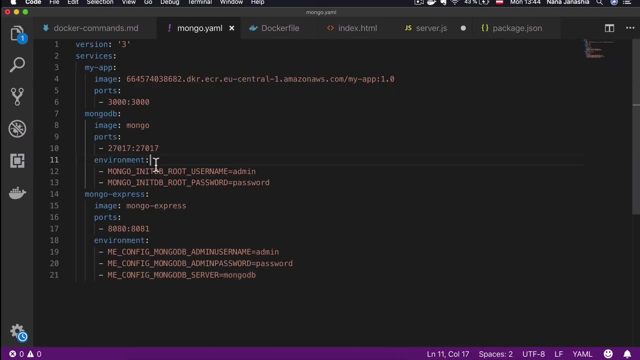 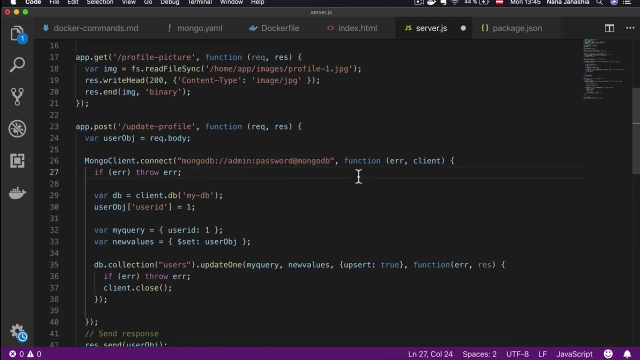 No, any more. actually, I wouldn't even need to use the port, even because I have all that information, So the host name and the port number, in that configuration. so my application will be able to connect to MongoDB using the service name And because of that you don't have to specify here a local host and the port number, which is actually even more advantage when you consider using Docker containers. 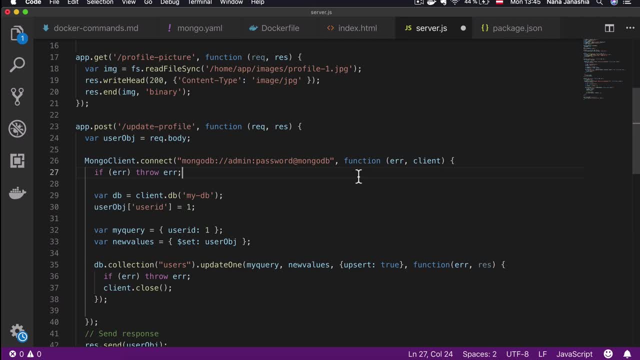 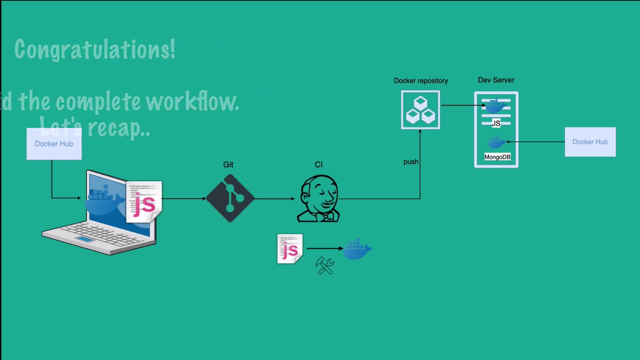 To run. run all of your applications, because it makes the connectivity between them even more easier. And that actually concludes this diagram that we saw previously. we have gone through all of the steps where we saw how to develop a JavaScript application locally with Docker containers. Then we saw how to build them into an image, just like a continuous integration.